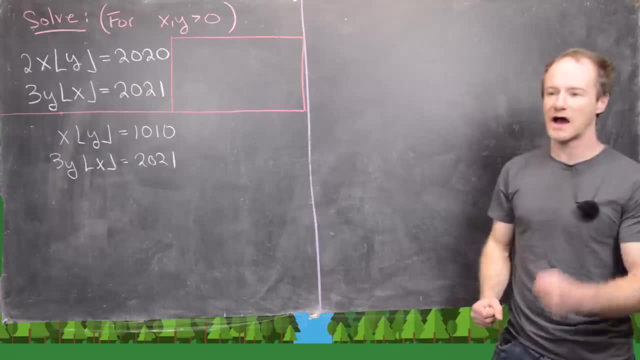 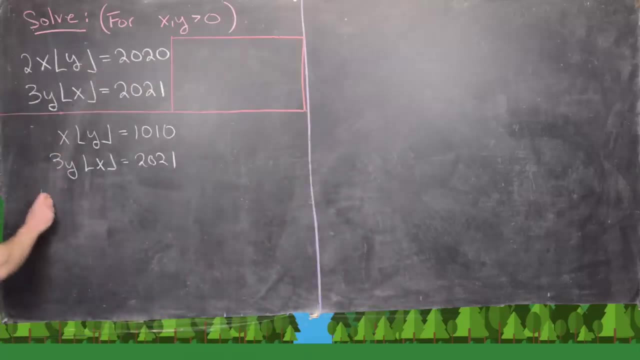 Now the next thing that I want to do is decompose x and y into their integer part and their fractional part, and I'll do that in the following way. So we're going to go ahead and write: x equals the floor of x plus a, and here a is going to be on the interval 0 to 1.. So notice if 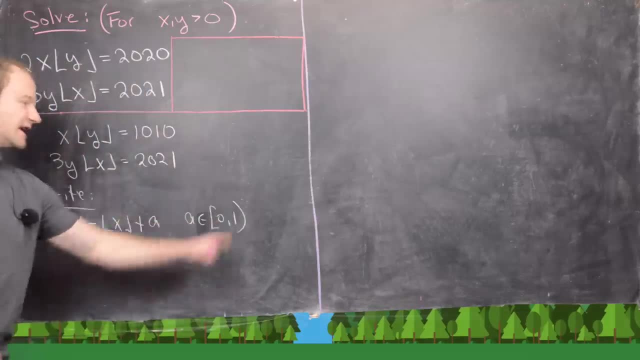 x is already an integer, then a is equal to 0, but then it can go all the way up to 1, but not include 1.. And then, furthermore, we'll say y is equal to the floor of y plus b, and here b is: 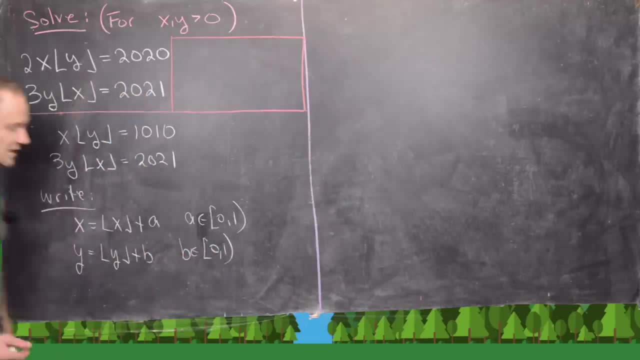 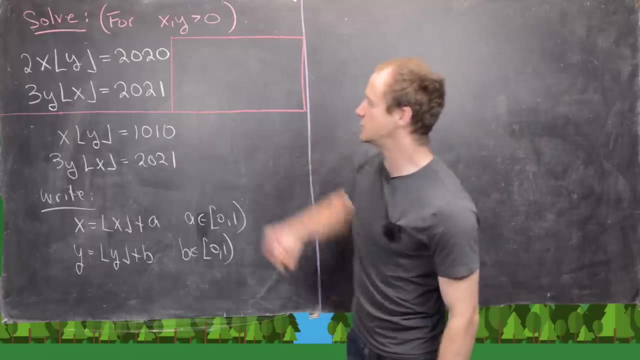 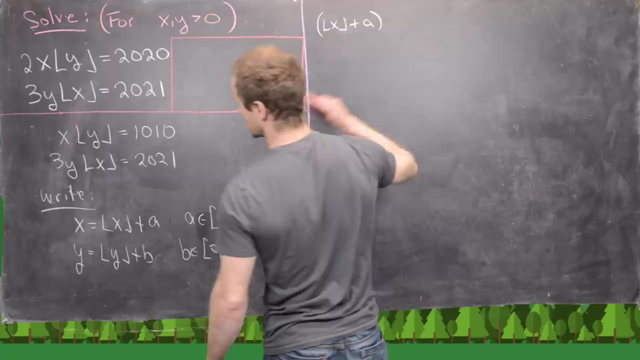 also going to be between 0 and 1.. Okay now, the next thing that I want to do is divide this thing, is take this realization of x and y and put it into our system of equations. So let's see what we get when we do that. So we're going to have the floor of x plus a times the floor of y, equals. 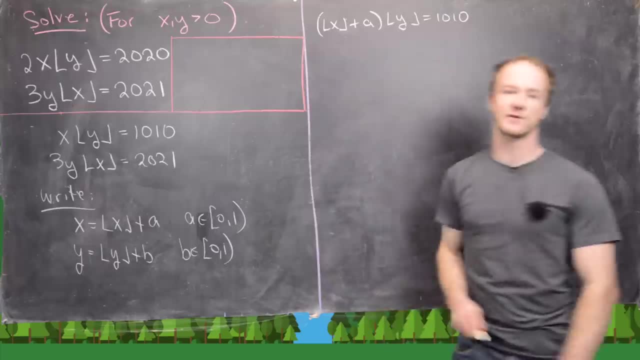 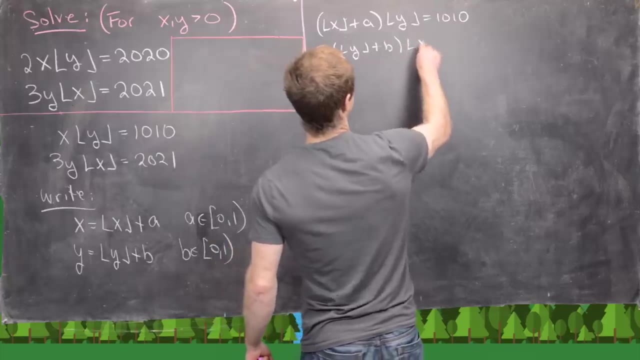 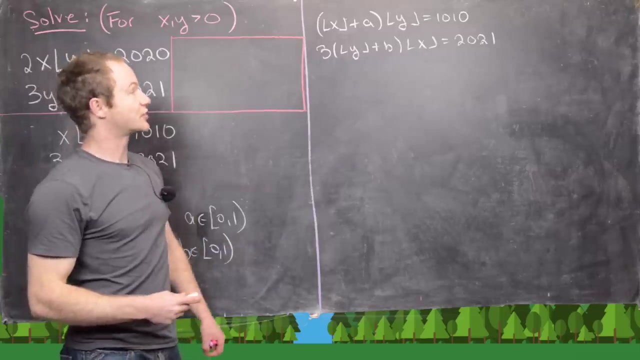 1010.. So that's what we get from plugging this into the first equation, And then we're going to have 3 times the floor of y plus b times the floor of x equals 2021.. Great. Now what I'm going to do is distribute that as much as I can, So that's going to give me. 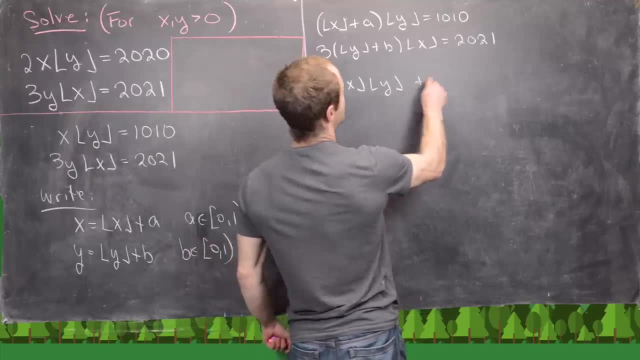 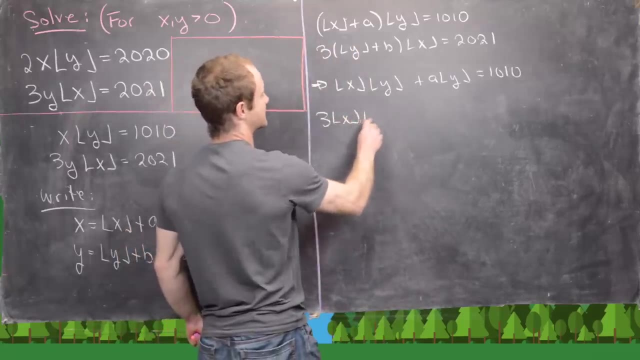 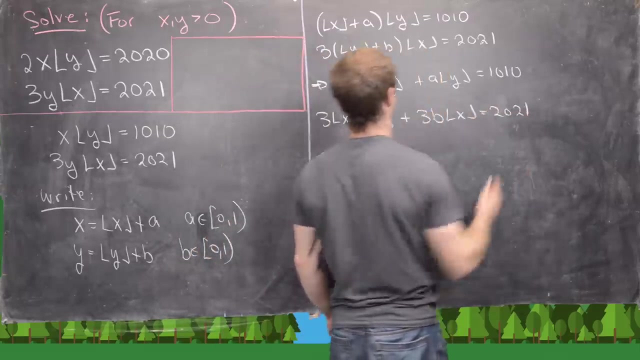 the floor of x times the floor of y plus a times the floor of y equals 1010.. And then I have 3 floor of x floor of y plus 3b floor of x equals 2021.. And this is actually maybe a little bit. 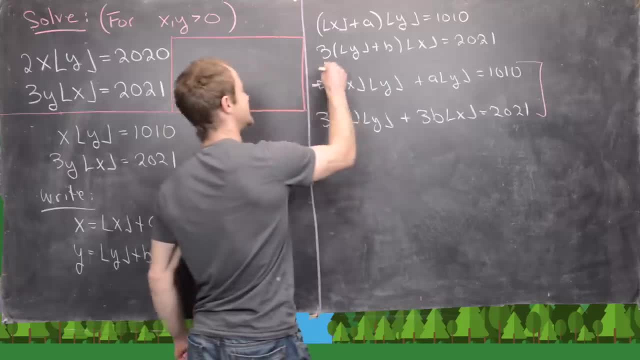 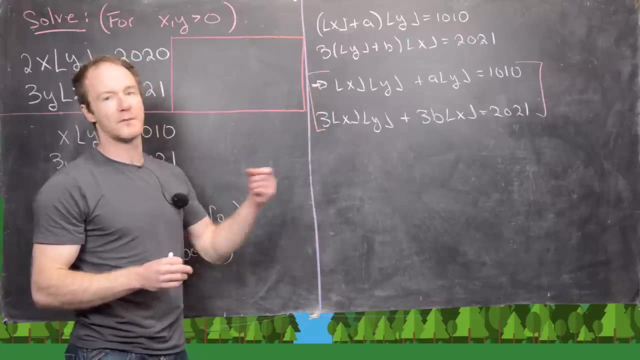 more helpful than it might seem, And that's because, if we're going to do this, we're going to take these two equations. we notice that two portions of each are integers and the remaining one portion is kind of unknown if it's an integer or not. So, for example, floor of x times floor of. 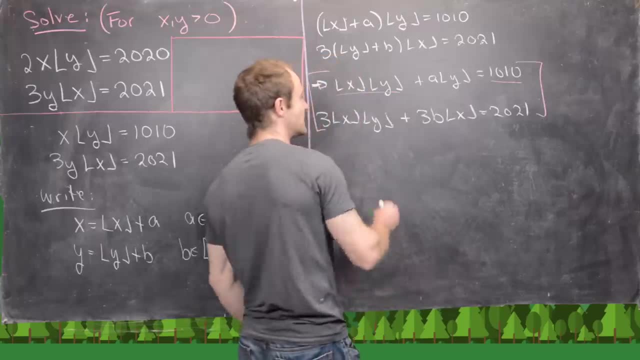 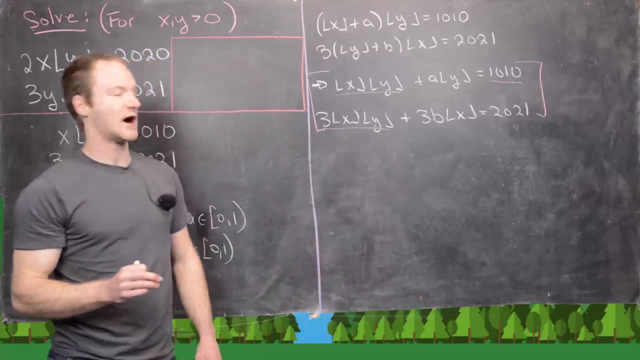 y is an integer and 1010 is an integer, but that tells us that a times floor of y is an integer, And likewise, 3 times floor x floor y is an integer. 2021 is an integer. that tells us that. 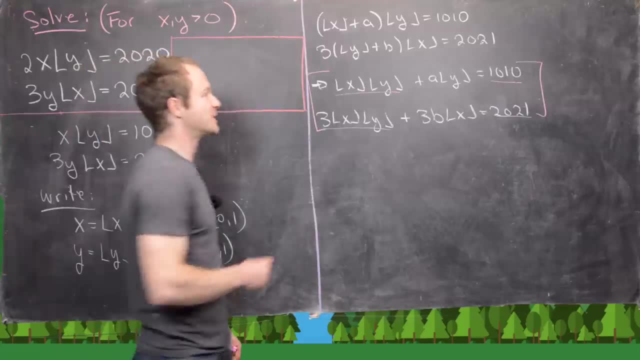 this: 3b times floor of x equals 4b. times floor of y equals 4b, And so we're going to have a. x is an integer, Okay, so just to be really thorough, that means that we can write a times: 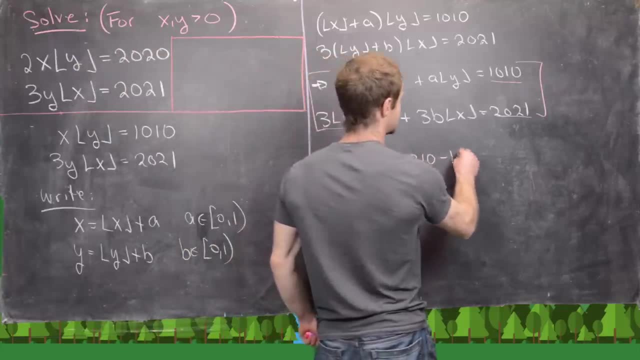 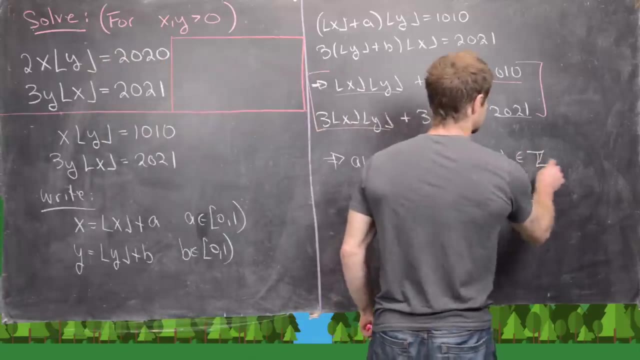 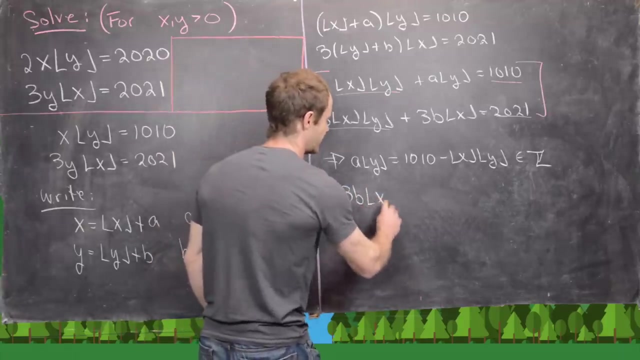 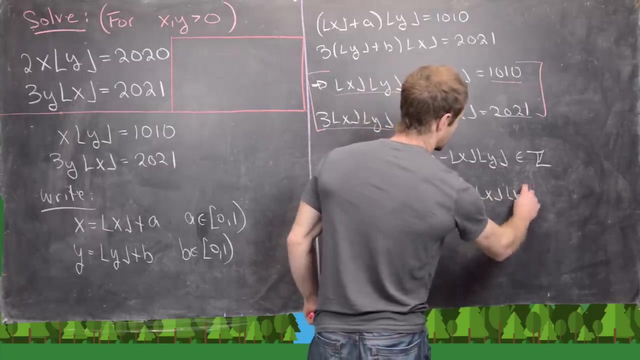 the floor of y equals 1010 minus floor x floor y. but we've got a combination of integers on the right-hand side, so we know that this is an integer. We can do the same thing for the second equation. That's going to give us 3b floor x equals 2021, minus 3 floor x floor y. That is also an. 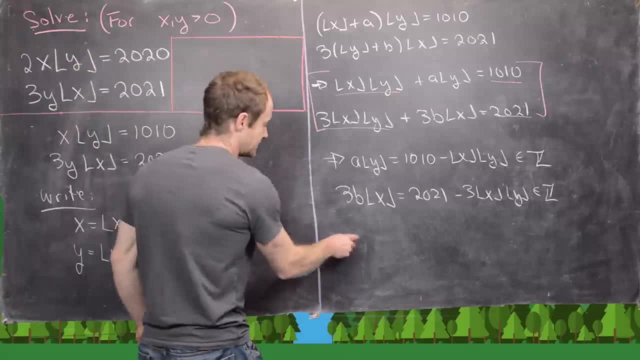 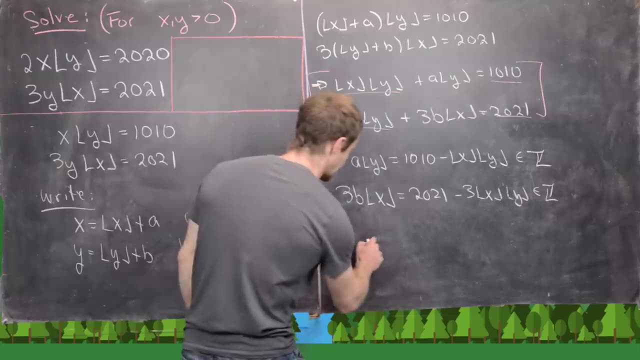 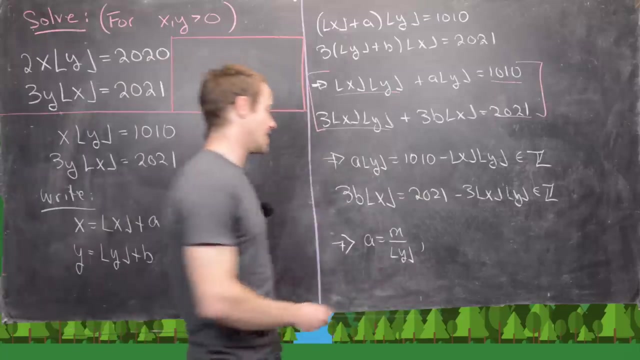 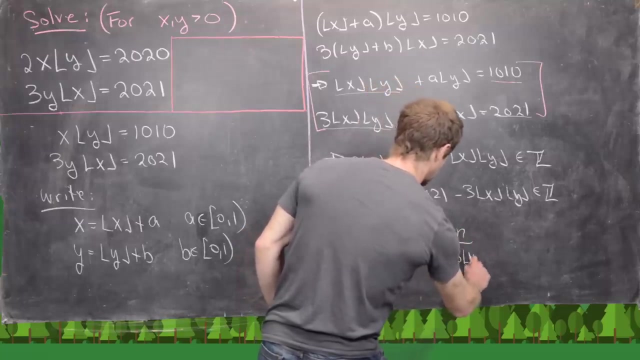 integer, Great. but what that tells us is that we can write a as a quotient involving the floor of y. In other words, we can write: a is equal to m divided by the floor of y, and similarly, we can write b As n divided by 3 times the floor of x. And how did we do that? Well, we know that these are. 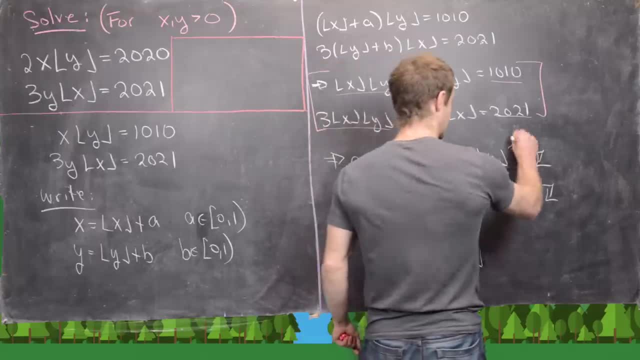 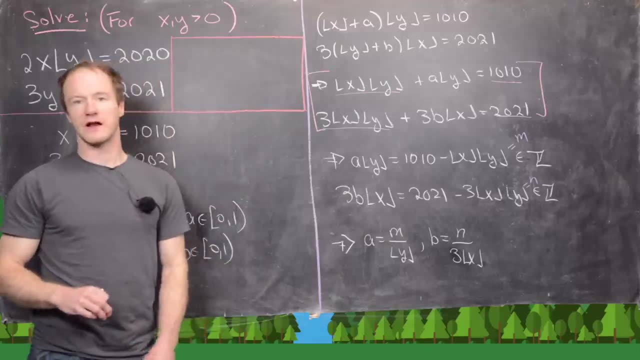 integers, and so we just give those integers names. We would give this the integer name m, and then we would give this the integer name n- Okay, great. And then by an argument, you know that those are not going to be equal to zero. so that's actually pretty easy to see. So now the 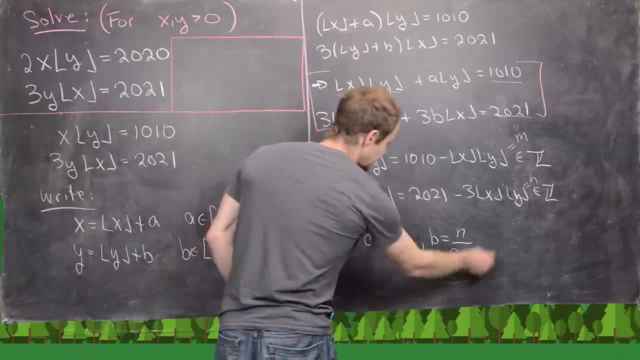 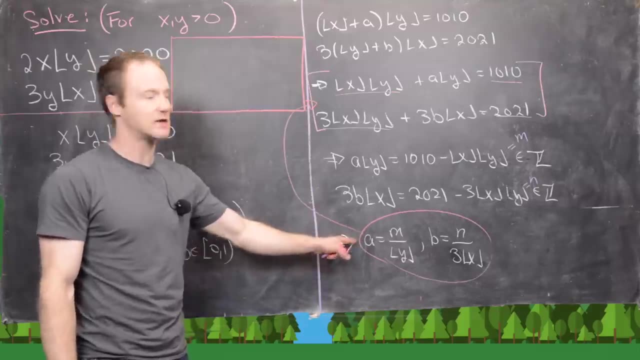 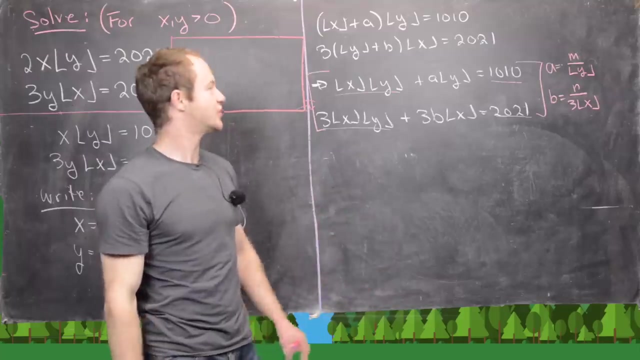 next thing that we want to do is loop these two values of a and b into this system of equations. Okay, so let's go ahead and loop this into this system of equations. I'll put the result right here and then we'll continue on. Okay, so we just noticed that this 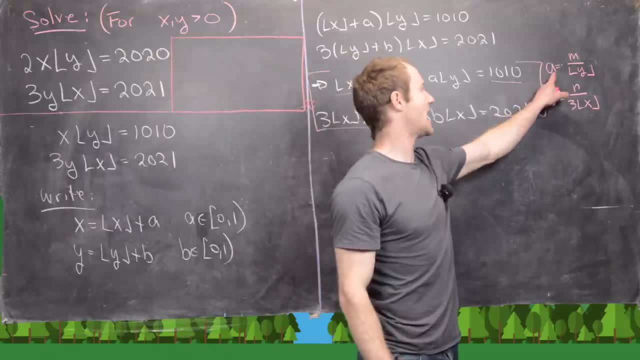 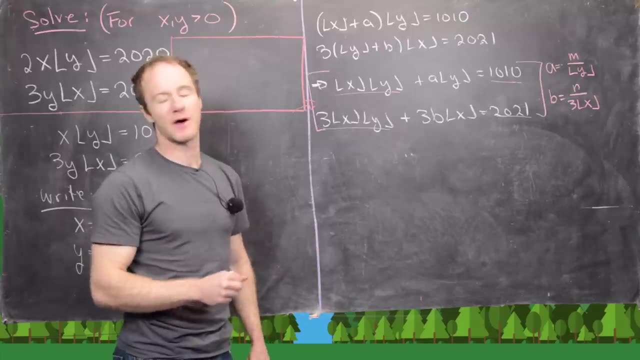 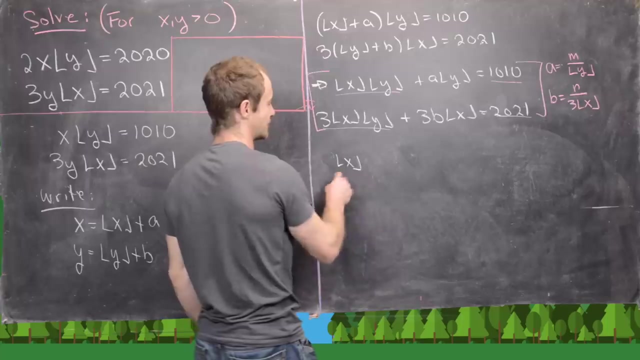 number a and this number b are of the following form: A is equal to an integer m divided by the floor of y, and b is equal to an integer n divided by three times the floor of x. Now, looping that into this system of equations gives us the following simplification we have: 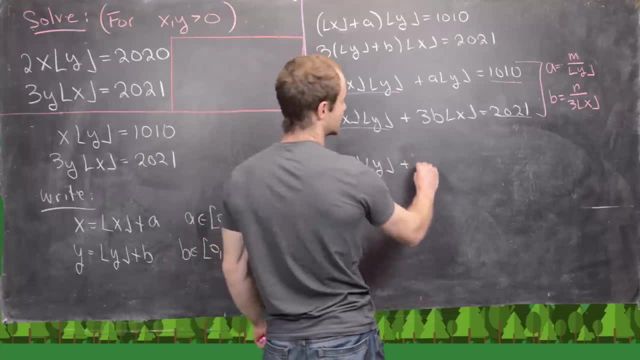 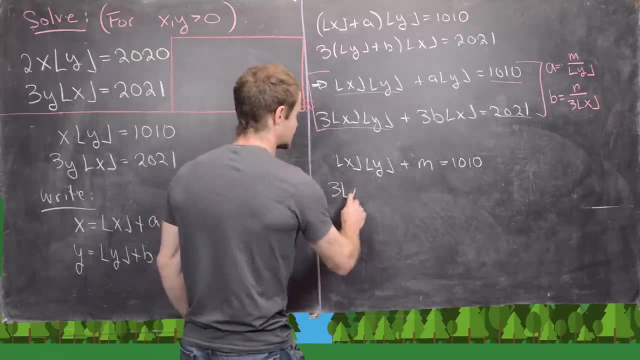 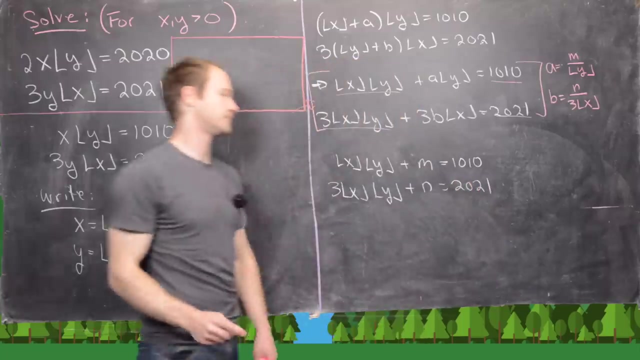 the floor of X times the floor of Y plus now this is just: M equals 10: 10, and now we're gonna have 3 times the floor of X, times the floor of Y plus N equals 2021. okay, fantastic. now, from here, what we want to do is cancel the floor of X and 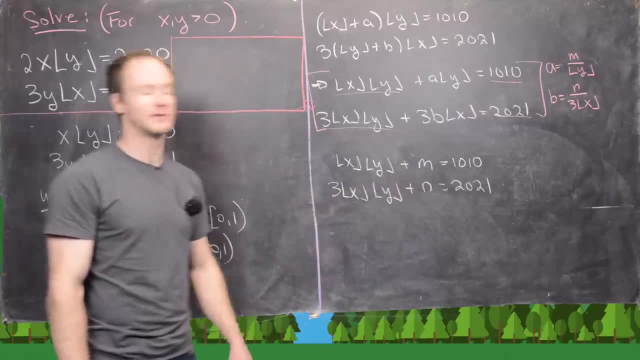 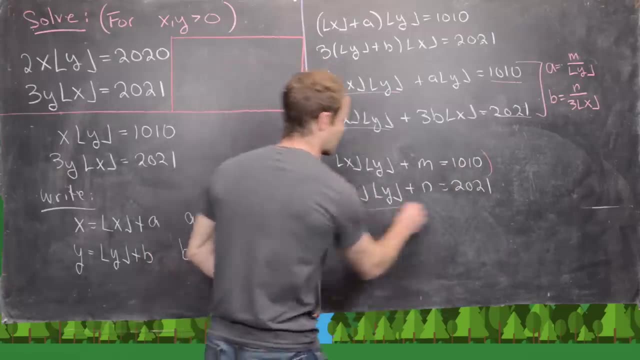 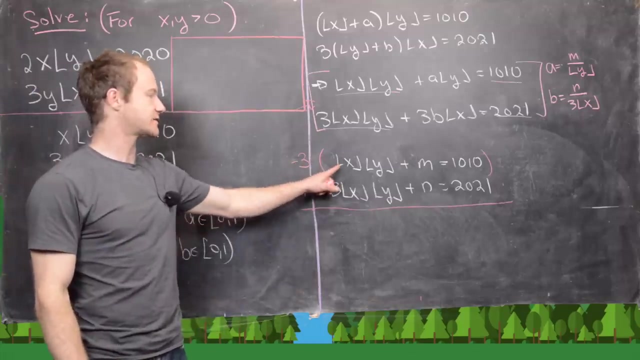 floor of Y term. so we get some sort of relationship between M and N. and we can do that by taking this first equation, multiplying by negative 3 and then adding them. so let's see what we get. when we do that, we've got minus 3 times. 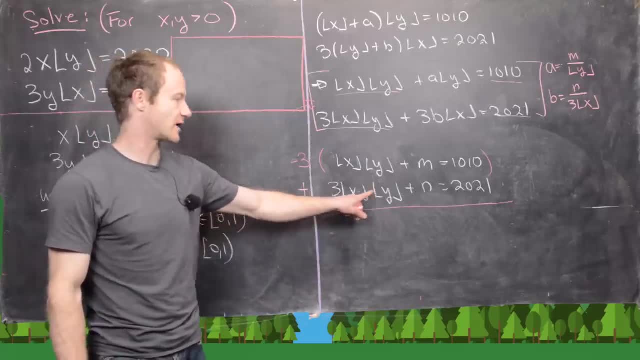 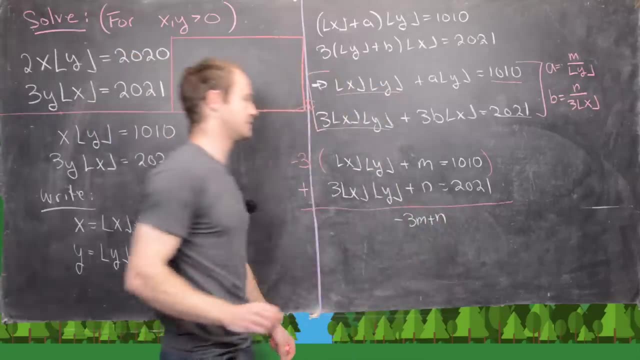 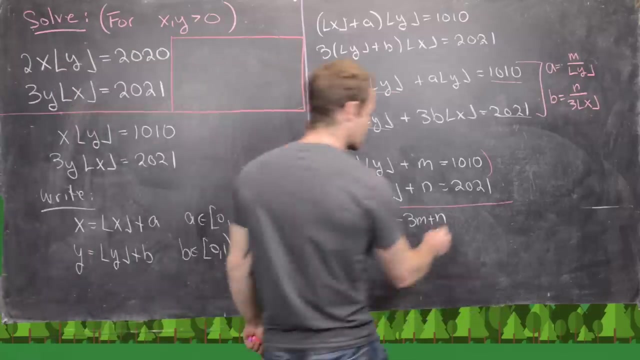 4 X times 4 Y, plus 3 times 4 X times 4 Y. so those are going to cancel, and then we're going to have minus 3 M plus N, and then we're going to have minus 30, 30 plus 2021. so that's going to give us minus 1009. so now we can rewrite. 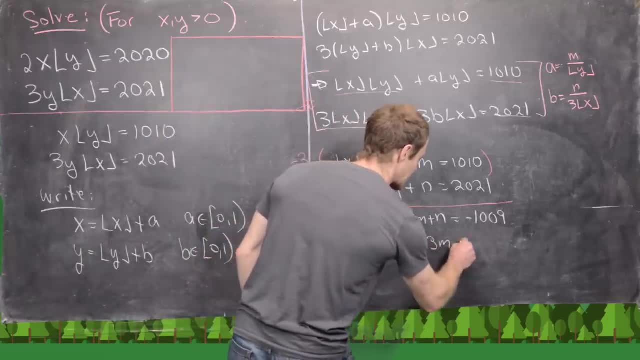 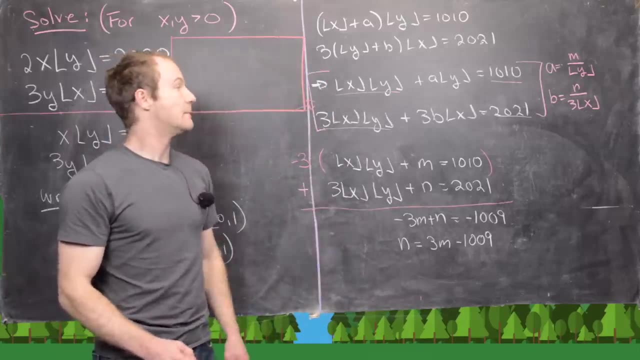 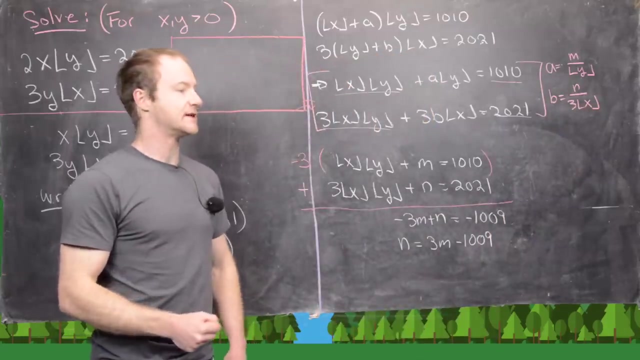 this a little bit and we'll see that N is equal to 3 M minus 1009 and that that may not seem super helpful at the moment, but remember our assumption is that X is a positive number, which means the floor of X is bigger than or equal to zero. I. 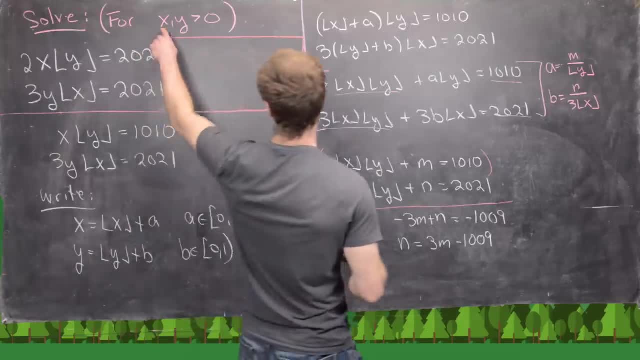 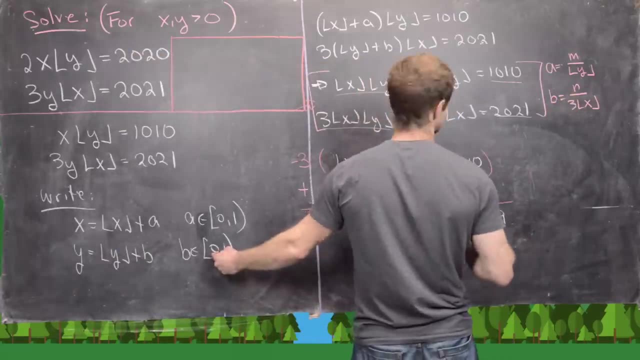 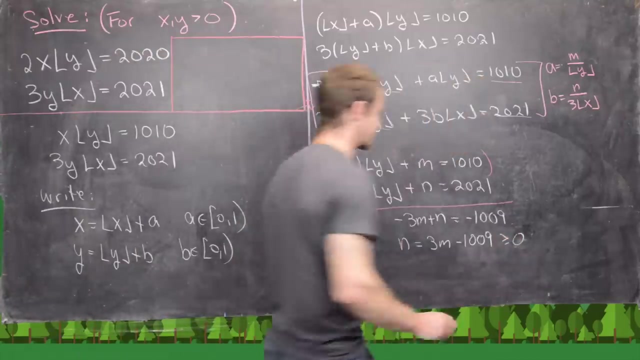 mean, obviously, if we're dividing by the floor of X, we've already assumed that the floor of X is bigger than or equal to one. also, we have: B is positive, which makes N a positive number. so that means we can say that this is bigger than or. 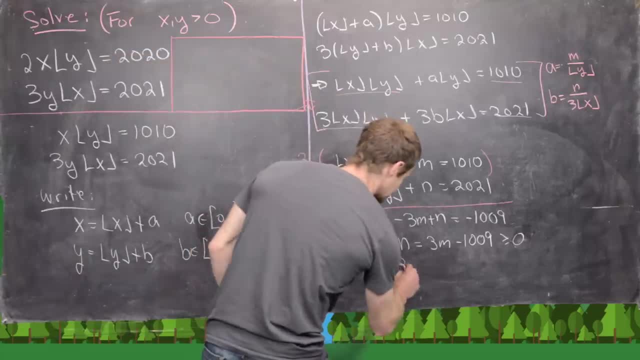 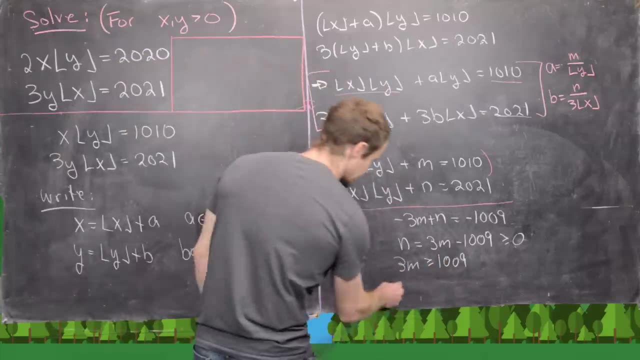 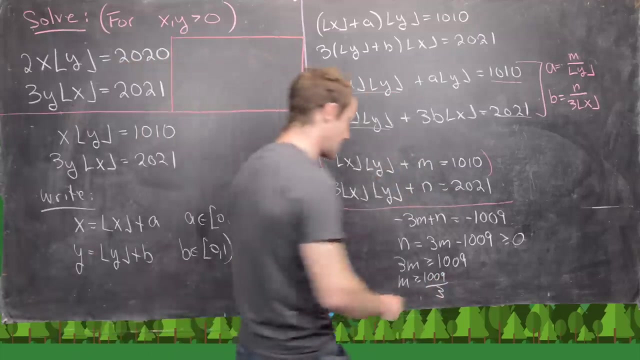 equal to zero. okay, good, but that's going to tell us that 3M is bigger than, or equal to, 1009. but that tells us that M is bigger than or equal to, 1009 divided by 3. but since M is an integer, that immediately. 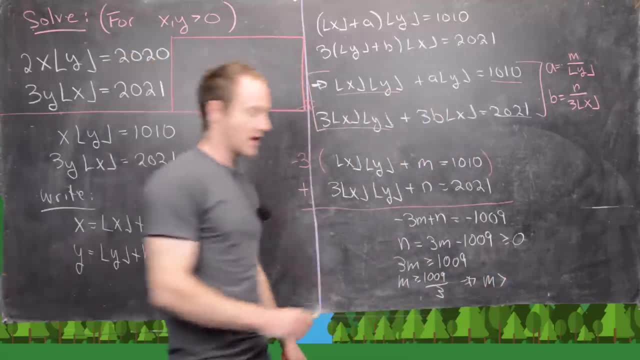 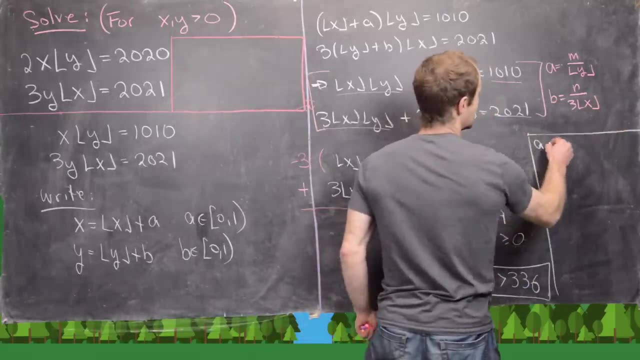 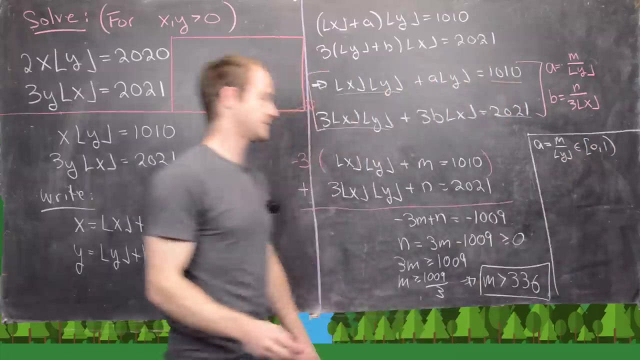 tells us that M has to be bigger than 336. so now let's see what that gets us. so we also know that A is equal to M over the floor of Y, and we know that that is in the interval 0 to 1. but that tells us that the floor of Y needs to be bigger than or equal to 0. so 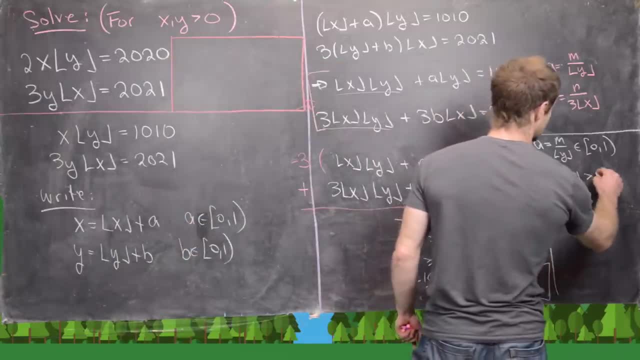 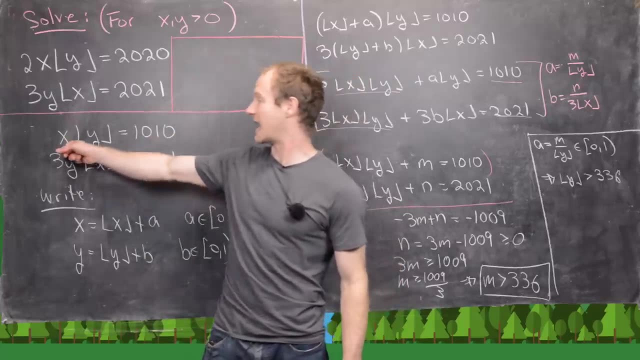 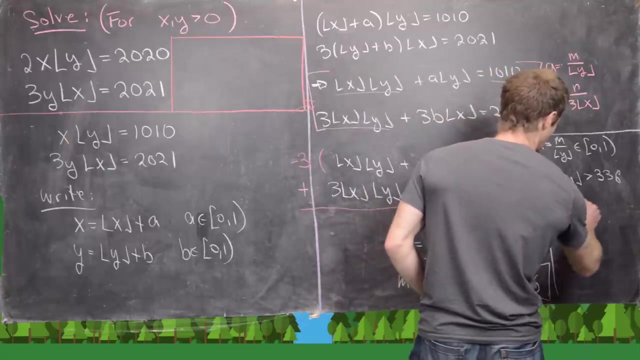 we know that the floor of Y is bigger than M, in other words, the floor of Y also needs to be bigger than 336. but now we also know from our original setup that X times the floor of Y is equal to 1010. so let's go ahead and write that over here: X times floor of Y is: 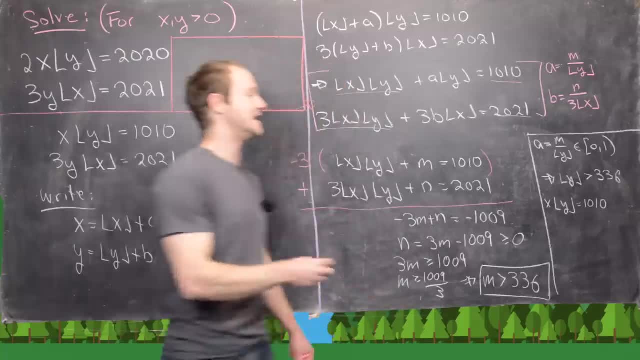 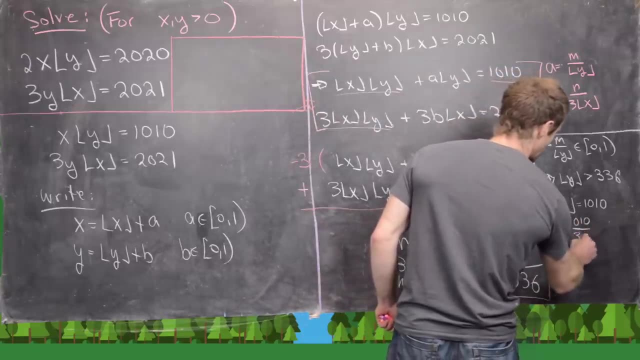 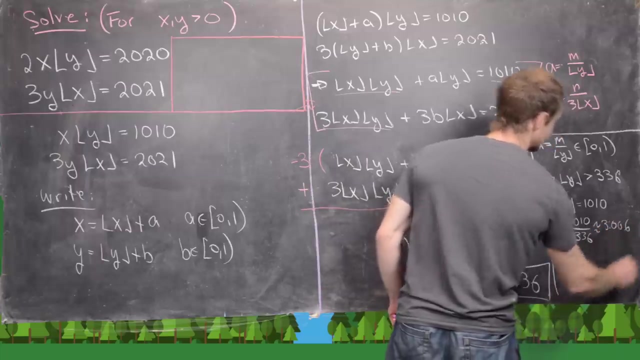 equal to 1010. but given the fact that Y is bigger than 336, that tells us that X needs to be less than 1010 over 336. which is approximately equal to 3.006. so still, X can be a ton of values, but the floor. 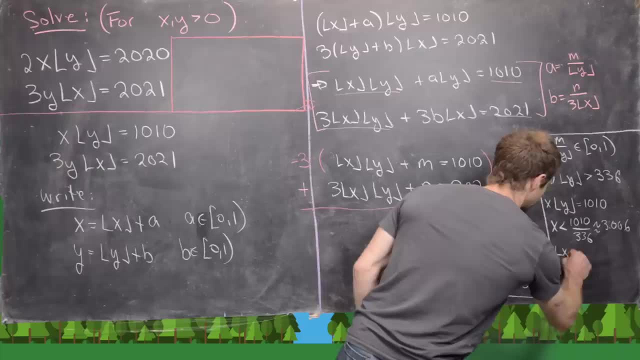 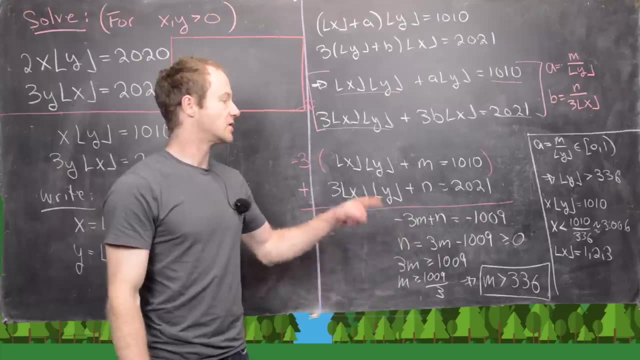 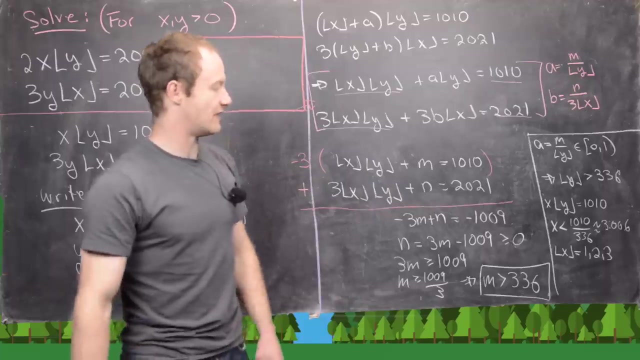 of X can only be a few things now. so notice that the floor of X, in this case, can only be one, two or three. okay, good, so let's go ahead and test each of those values. so I'll clean up this part of the board and then we'll test each of those values of the floor of 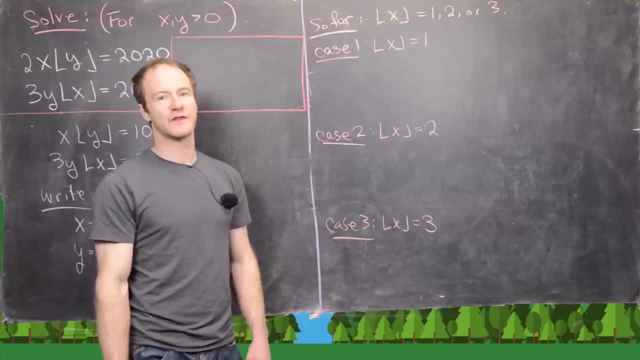 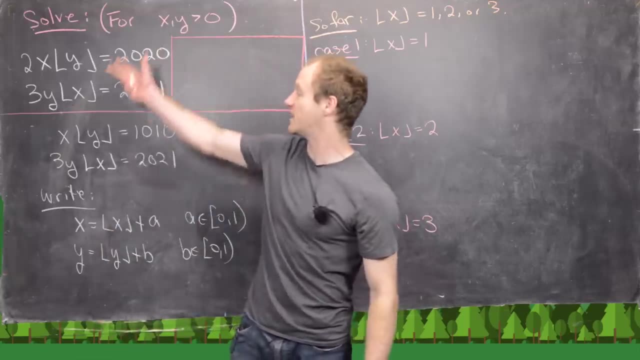 X one, two and three. so we just got done arguing that the floor of X can only take on the values one, two or three, and we can use that to our advantage to actually finish solving this system of equations right here. so let's look at this first case, when the floor of X equals. 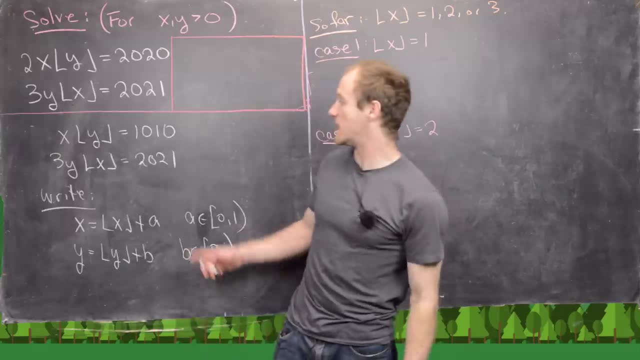 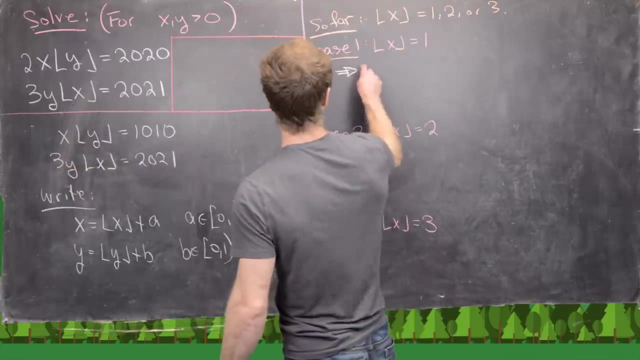 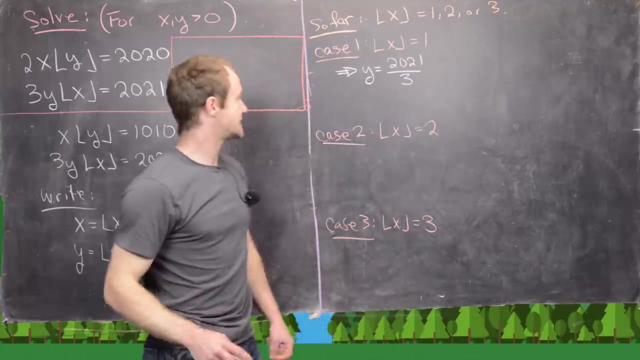 one. so plugging the floor of X equals one into this equation right here, three Y times the floor of X equals twenty twenty one. that immediately tells us that Y equals one. so that equals twenty twenty one over three. okay, fantastic. but now what we want to do is take 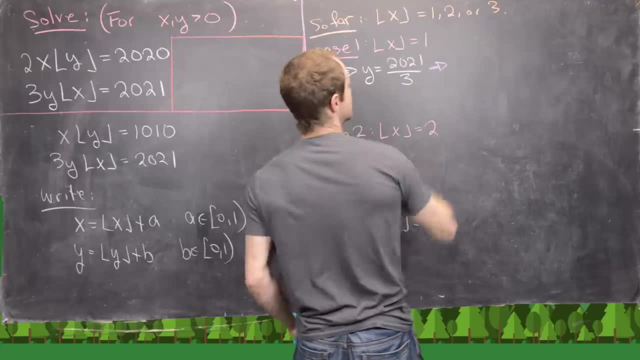 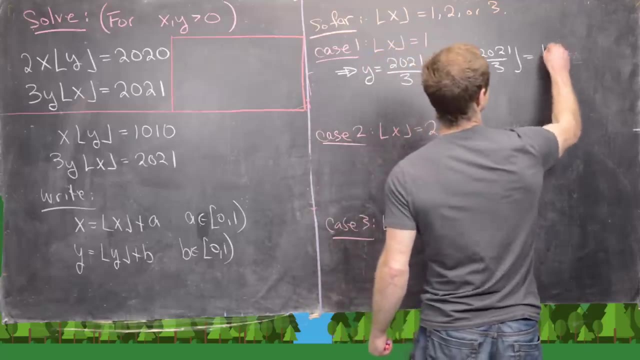 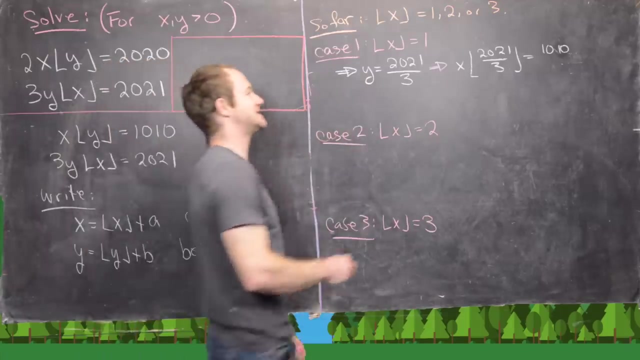 that and plug into this equation. so we have X times the floor of 2020, one over three equals 1010, but then you can check that the floor of 2020 one over three is 673. so let's just go ahead and point that out here. 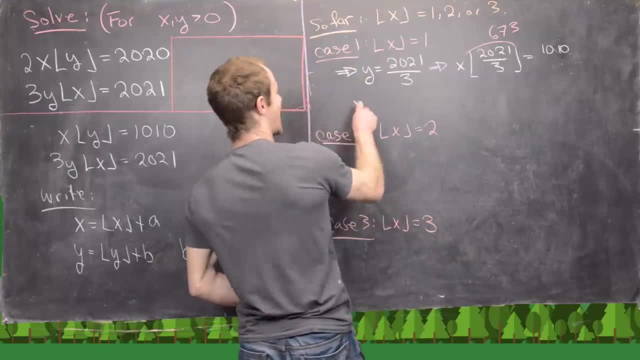 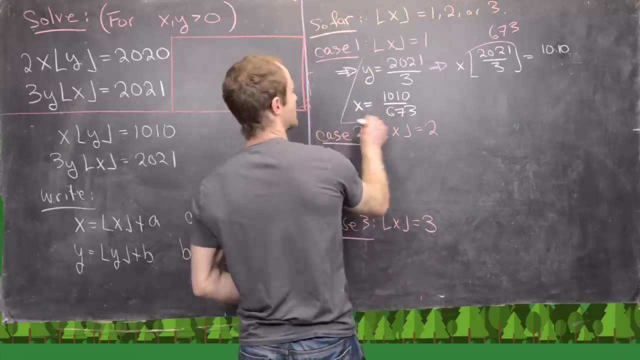 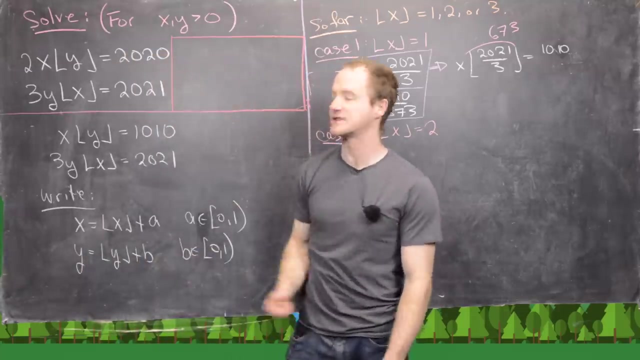 This is 673.. 673, which means x equals 10, 10 divided by 673. and then maybe, if you want to be real safe about it, you can just go ahead and plug these two values of x and y back into our original system and 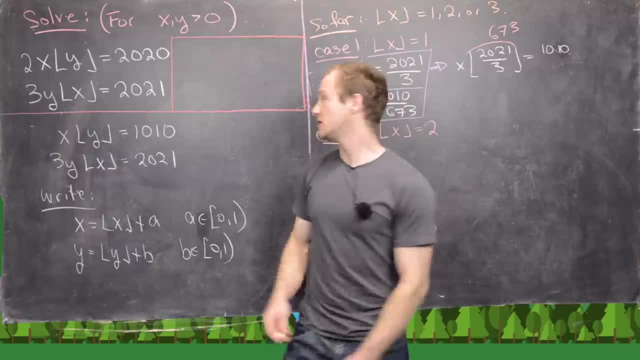 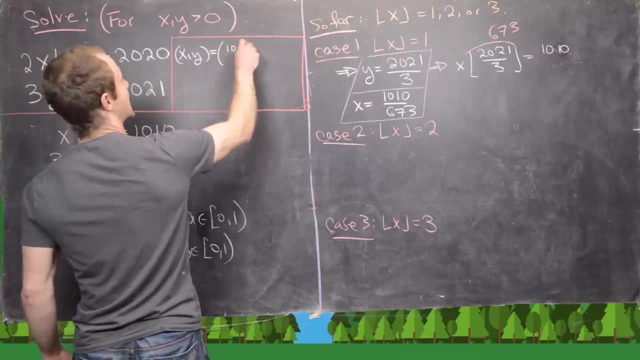 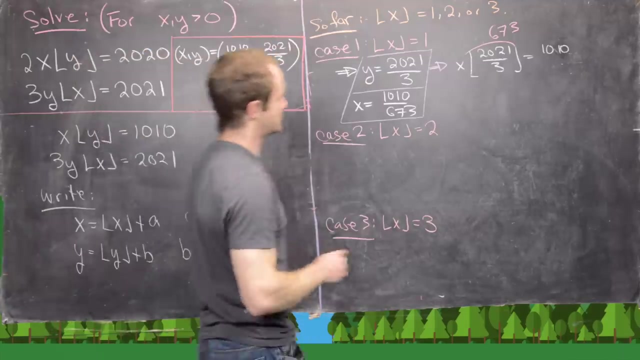 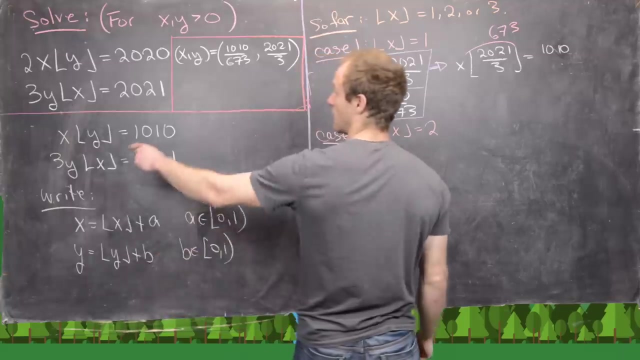 notice that the system is satisfied in this case. so let's go ahead and say that we've got one solution: x y equals 10, 10 over 673, comma 2021 over three. great, now let's see if we can get two more solutions. so let's say that floor of x equals two. so now plugging that into this equation, right?